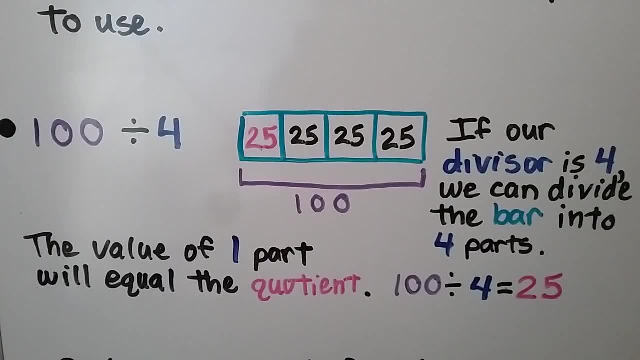 operation to use. Here we have 100 divided by 4.. Our bar model represents the 100 for the full bar and we can break it into four equal parts. If our divisor is 4, we divide the bar into four parts And the value of one part will equal the quotient. 100 divided by 4 is equal to 25.. So remember when 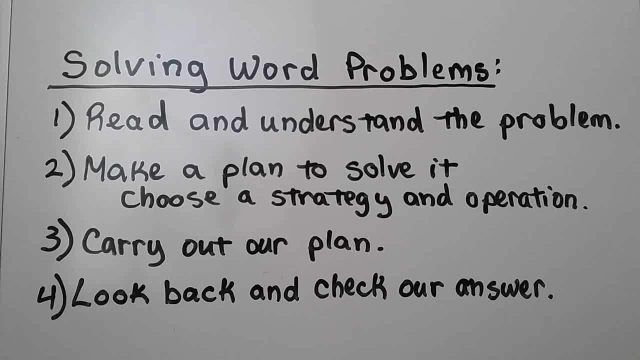 we're solving multi-step division problems. we're going to use the strategy, draw a diagram to solve word problems. One: we read and understand the problem. We make sure we know what it's asking us to find. Two: we make a plan to solve it. We choose a strategy and an operation Are we going to use? 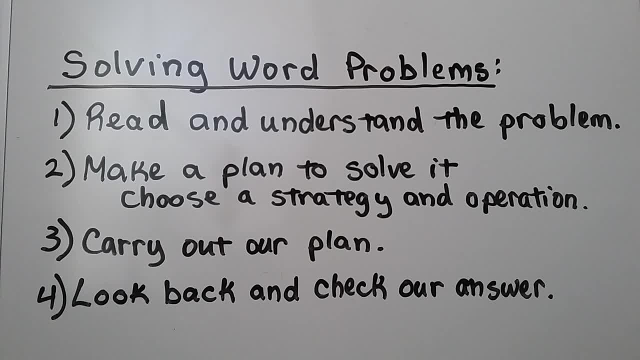 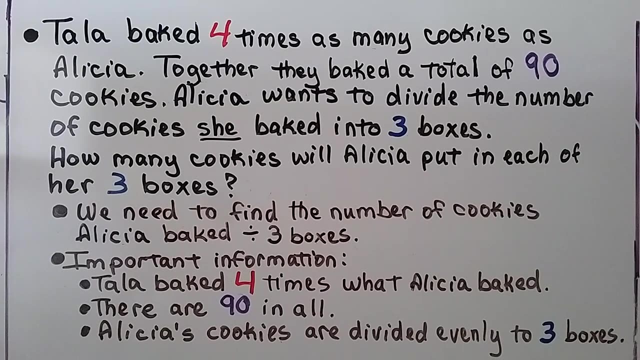 addition, subtraction, multiplication or division. Number three: we carry out our plan. And number four: we look back and check our answer. Tala baked four times as many cookies as Alicia Together. they baked more cookies. Alicia wants to find a total of 90 cookies. Alicia wants to divide the number of cookies she baked into three. 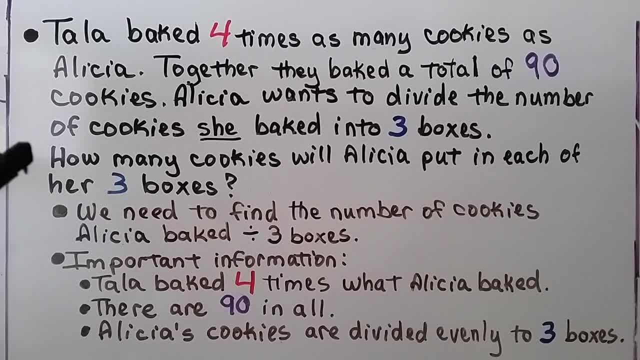 boxes. How many cookies will Alicia put in each of her three boxes? So we need to find the number of cookies that Alicia baked. We need to divide it into three boxes. Our important information is that Tala baked four times what Alicia baked. There's 90 in all. There's 90 cookies all together And Alicia's. 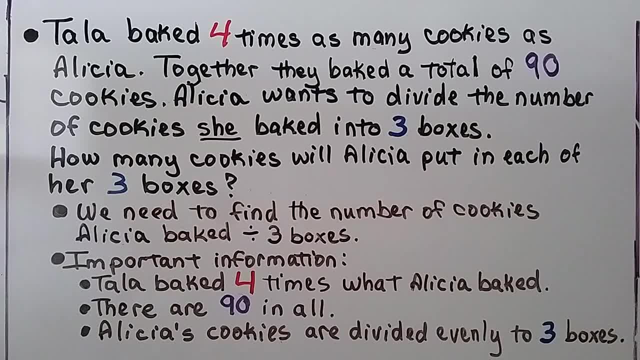 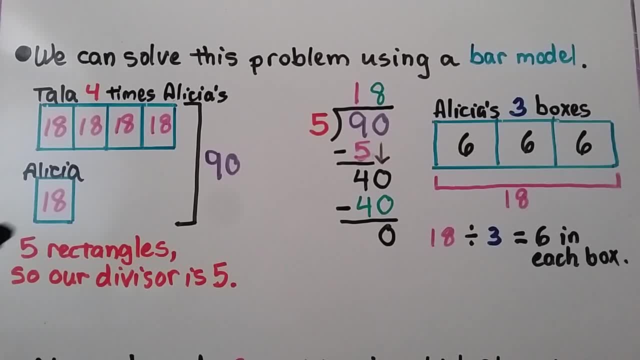 cookies are divided evenly to 30.. Alicia's cookies are divided evenly to 30.. Alicia's cookies are divided evenly to three boxes. We can solve this problem using a bar model. We know we need to find Alicia's amount that she baked and that Tala is four times Alicia's, So we make one. 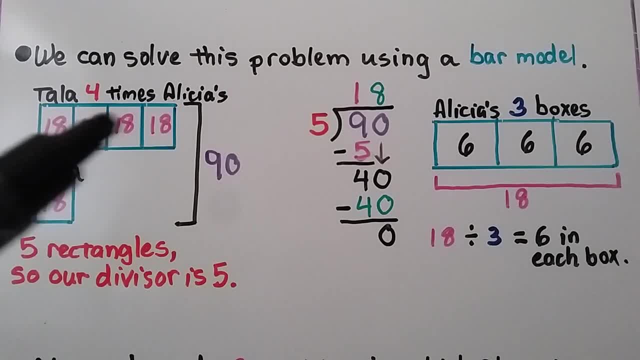 rectangle for Alicia's amount and four for Tala's, Because she's four times Alicia is one. Four times one is four. So we have five rectangles, five parts. So our data should be relevant to the paste in Хот. Now. 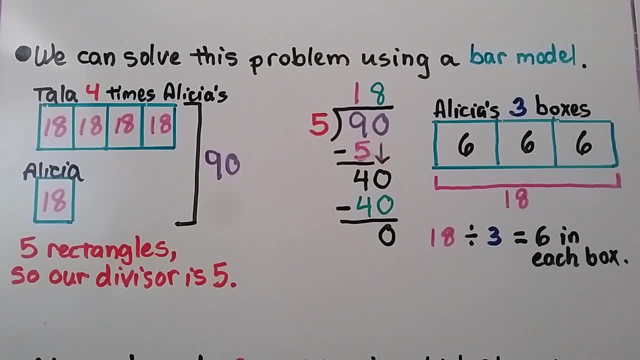 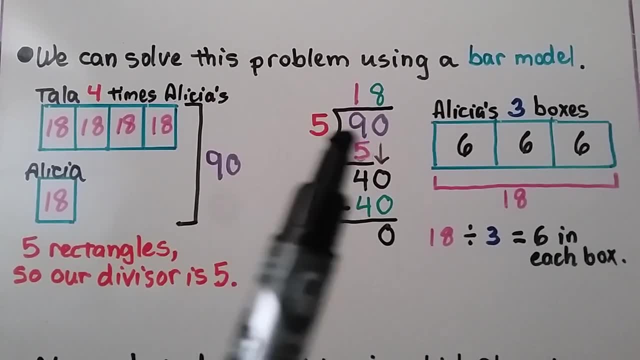 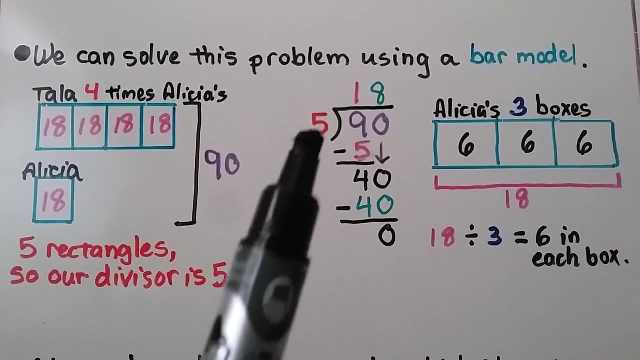 divisor is going to be 5.. We know they baked 90 in all. We can do 90 divided by 5.. We ask ourselves: how many times can 5 fit into 90?? 5 can fit into 9. one time We put a 1 above the 9 and 5 times 1. 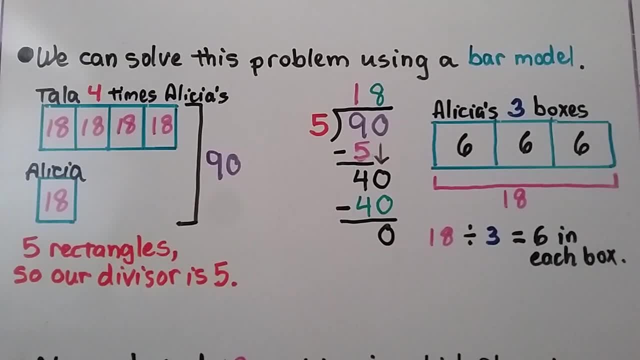 is 5 and we subtract that 5.. We get 4.. Now it's the zeros turn to come down and we ask ourselves how many times 5 can fit into 40? 5 times 8 is 40.. We put an 8 in our quotient and 5 times 8 is 40. 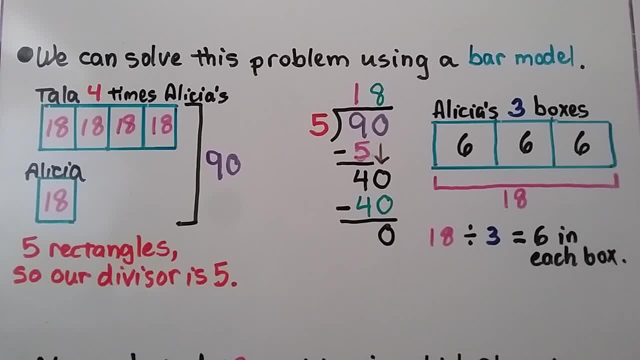 so that's what we subtract. We get a 0.. We know that Alicia baked 18 cookies. She needs to divide them into three boxes. We can make a bar model representing 18 in all and making three rectangles for the three boxes. 18 divided by 3 is equal to 6 in each box. 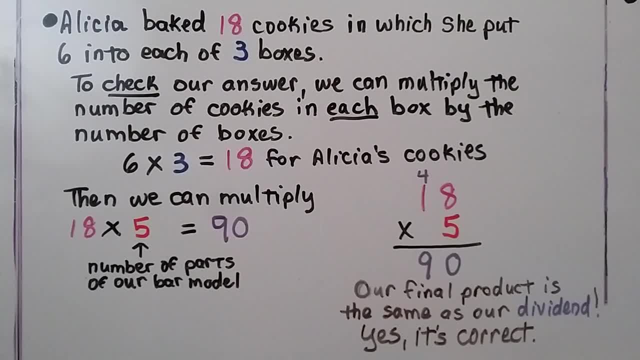 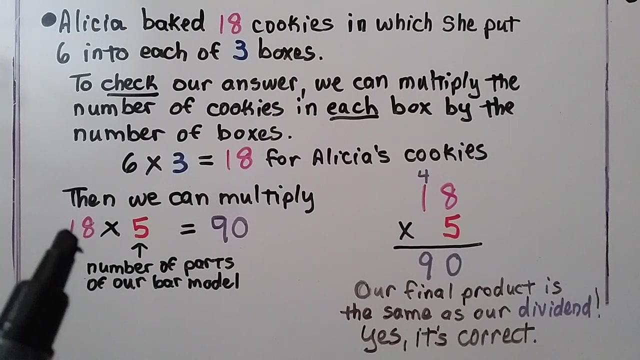 Alicia baked 18 cookies, in which she put 6 into each of three boxes. To check our answer, we can multiply the number of cookies in each box by the number of boxes. There were 6 in each box. She has three boxes. That's 18 for Alicia's cookies. That's correct. Then we can multiply the 18 that Alicia 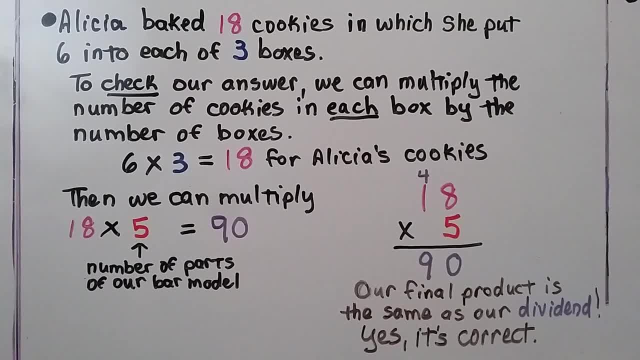 made times 5, which was the number of parts of our bar model. It's equal to 90.. 18 times 5, we do 5 times 8, which is 40. We regroup the 4 and put the 0 down. 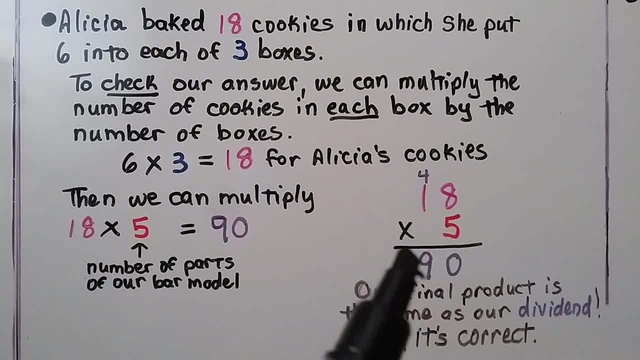 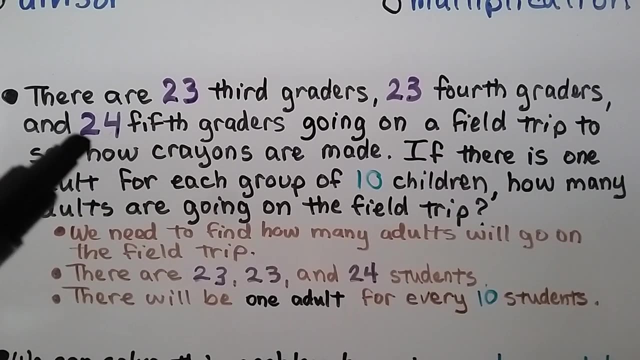 5 times 1 is 5 plus the 4 that we regrouped is 9.. Our final product is the same as our dividend. so yes, it's correct, There are 23 third graders, 23 fourth graders and 24 fifth graders going on a field trip to see how crayons are made. 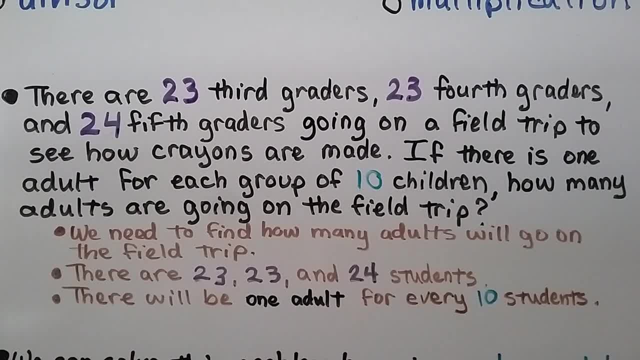 If there is one adult for each group of 10 children, how many adults are going on the field trip? We need to find how many adults will go on the field trip and we know there are 23,, 23, and 24 students. 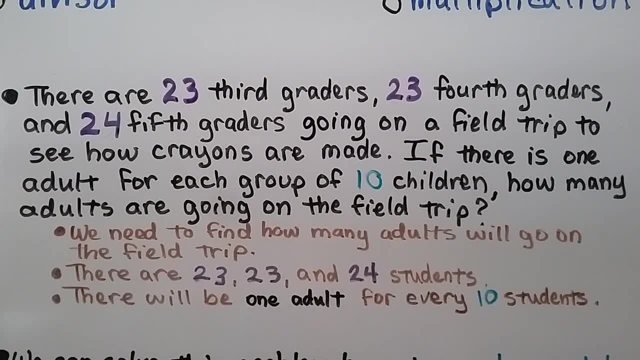 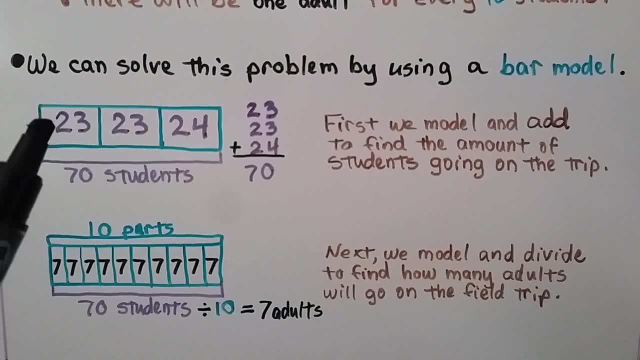 There will be one adult for every 10 students. We can solve this problem by using a bar model. we total it and get 70 students. So we model and add to find the amount of the students going on the trip. Next we model and divide to find how many adults will. 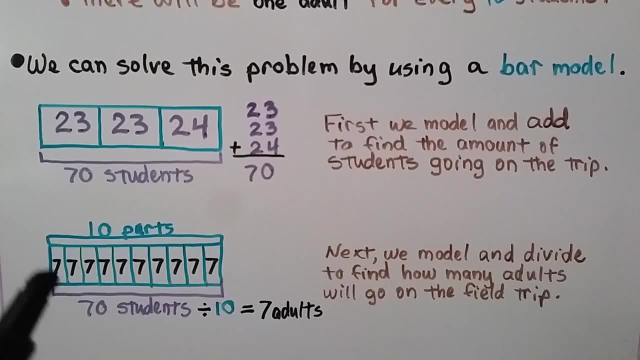 go on the trip. We know there's 70 students in all and we can make a bar with 10 parts, because there's going to be 10 children with each adult We get 7.. 70 students divided by 10 is equal to 7 adults. We can also use the equation: 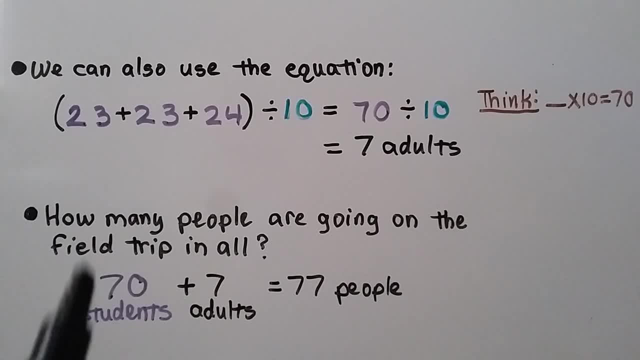 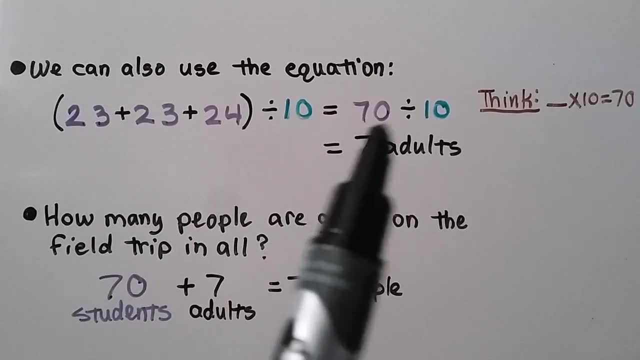 23 plus 23 plus 24 in parentheses. so we add them first divided by 10.. We add these, we get 70.. We do 70 divided by 10, that's 7 adults And we can think some number times 10 is equal to 70.. 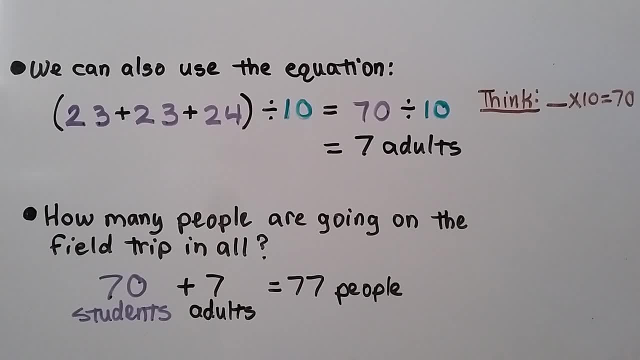 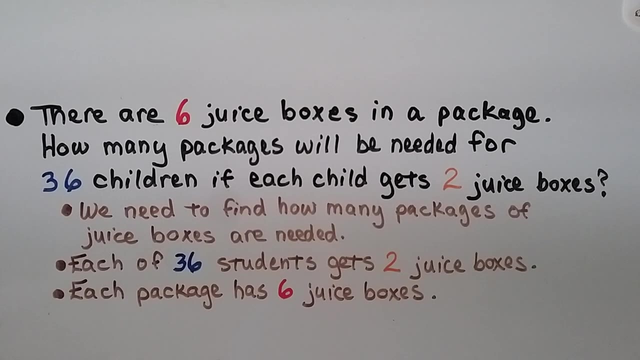 To help us solve it, And how many people are going on the field trip? in all, There's 70 students. There's 7 adults, That's 77 people. There are six juice boxes in a package. How many packages will be needed for 36 children if each? 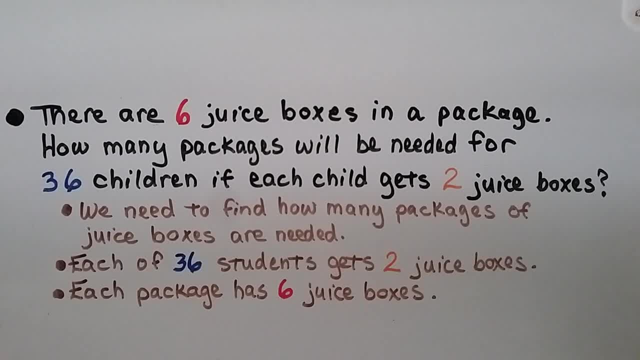 child gets two juice boxes, So we need to find how many packages of juice boxes are needed. Each of 36 boxes will be needed for 36 children, So we need to find how many packages of juice boxes are needed. Each of 36. 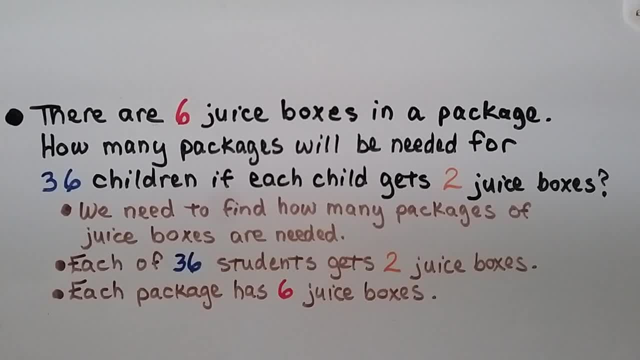 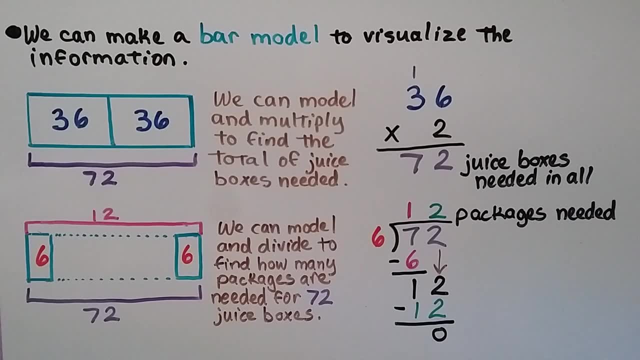 students gets two juice boxes and each package has six juice boxes. We can make a bar model to visualize the information. We have 36 children, students- and they're each going to get two juice boxes, so we can do 36 and 36.. 36 times 2 is 72. We do. 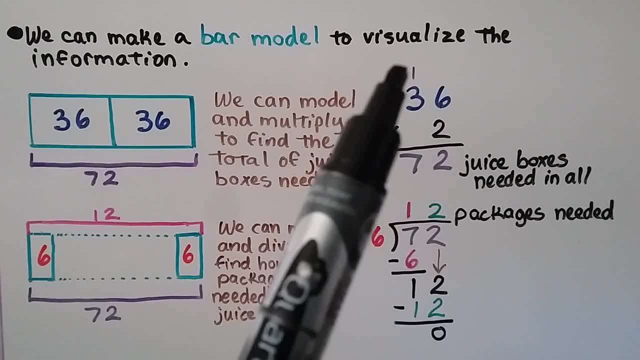 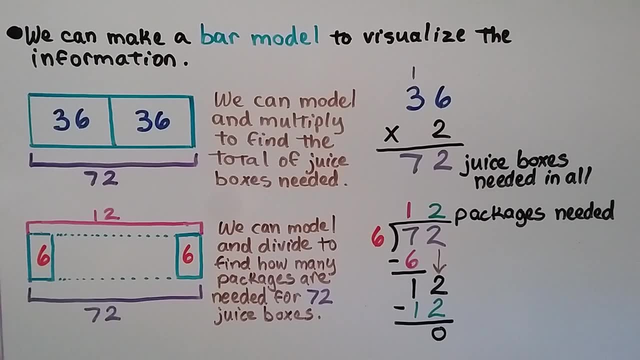 36 times 2.. 2 times 6 is 12.. We regroup the 1 and put the 2 down 2 times 3 is 6 plus the 1 we regrouped is 7.. So that's 72 juice boxes needed in all. 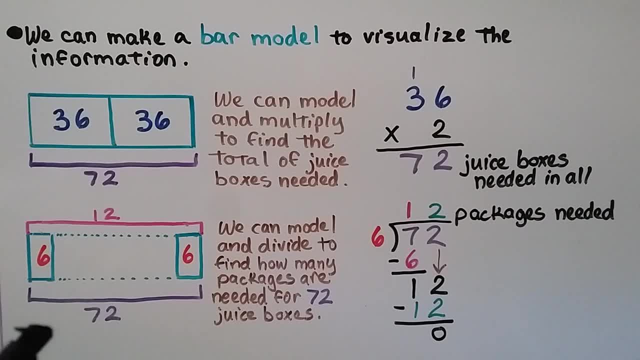 And we can model and divide to find how many packages are needed for 72 juice boxes. We know there's 72 needed in all. We know there's 6 in a package. We can make a bar model and fill it with rectangles of 6 until we have 72.. And we'll get 12.. 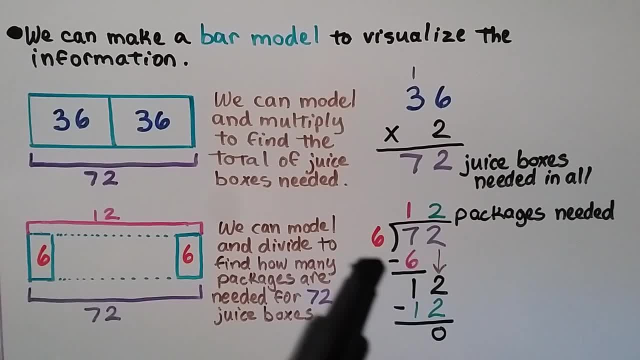 We can divide 72 divided by 6. 72 juice boxes needed by 6 in a package. We ask ourselves how many times the 6 fits into the 7.. That's one time We put a 1 above the 7. 6 times. 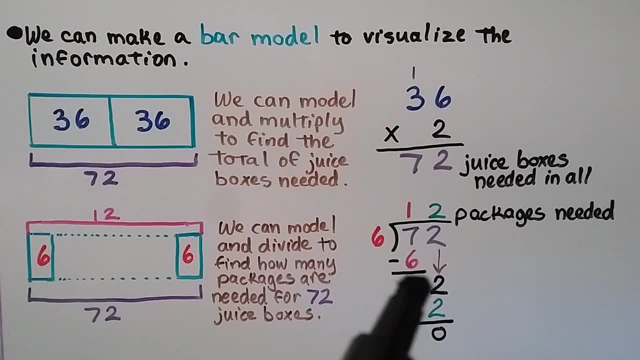 1 is 6, so we subtract it and get a 1.. We bring the 2 down. It's turned to come down. 6 fits into 12 two times, because 6 times 2 is 12.. We get it. We subtract it and get a 1.. We. 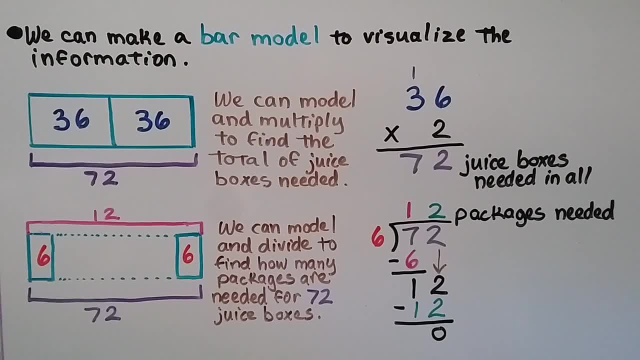 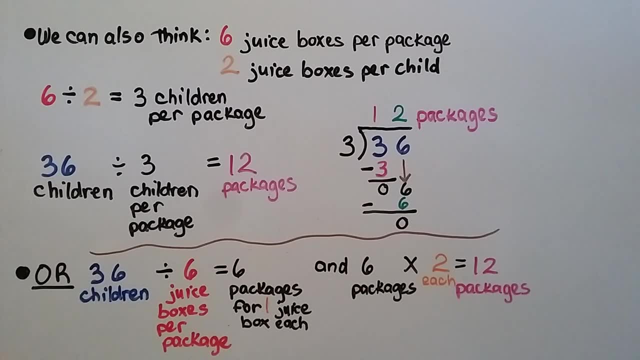 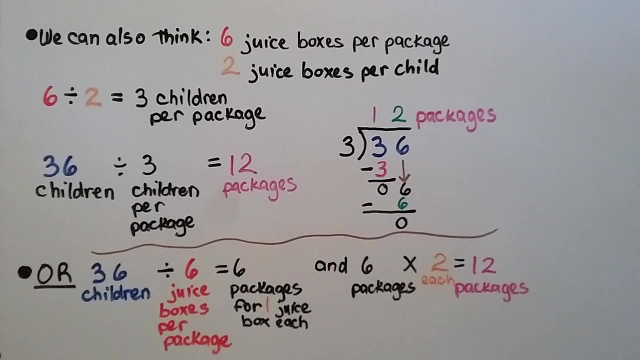 subtract it and get a 0 remainder. We know we need 12 packages of juice boxes. We can also think: well, 6 juice boxes per package, 2 juice boxes per child. That means 6 divided by 2 is 3 children per package. 3 children can get juice boxes per package. Then we can 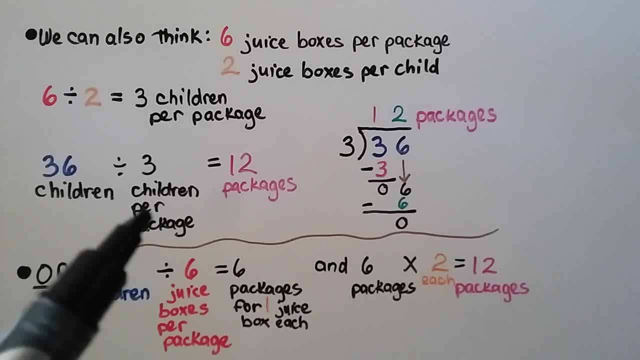 do: 36 children divided by the 3 children per package: 3 children divided by 2 is 7.. We need 1.. We subtract it, We get a 0. remainder: 0 packages of juice boxes needed. We know we need. 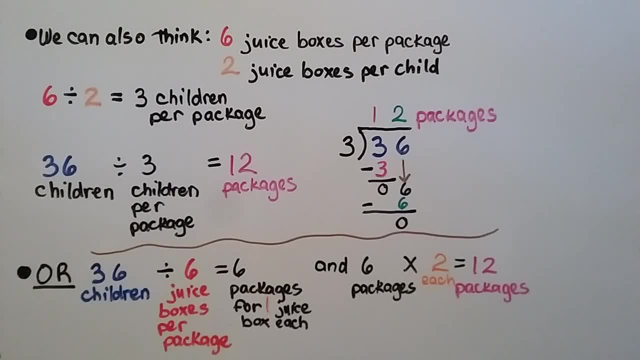 package and we get 12 packages. We can also think 36 children divided by 6 juice boxes per package is going to be 6 packages for 1 juice box each, but they're gonna have 2 juice boxes each, So we can multiply this 6 times 2 for 2. 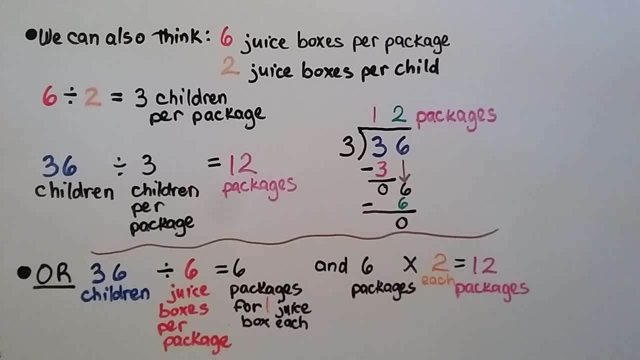 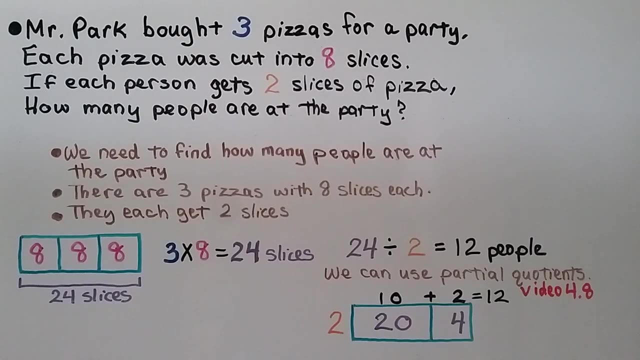 each and we get 12 packages. There's usually more than one way to solve a problem. it's just that some ways are more efficient and some ways are easier. Mr Park bought three pizzas for a party. Each pizza was cut into eight slices. If 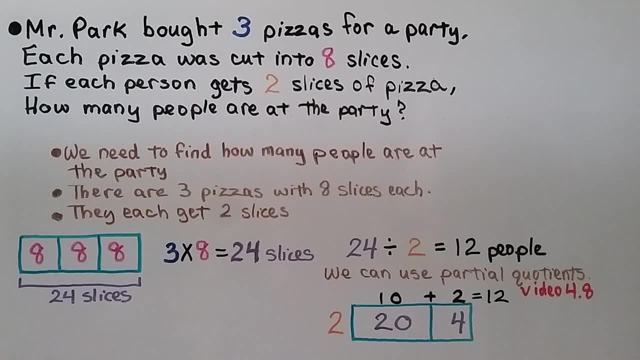 each person gets two slices of pizza, how many people are at the party? Mr Park bought three pizzas for a party. Each pizza was cut into eight slices. If each person gets two slices of pizza, how many people are at the party? 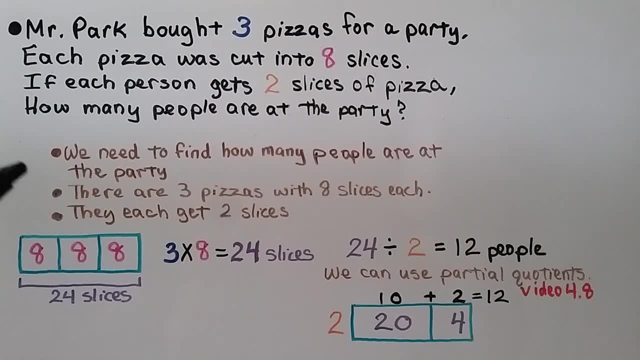 So we need to find how many people are at the party. There are three pizzas with eight slices each. They each get two slices. We can do 8 times 3 or 3 times 8 and we get 24 slices. So we know there's 24 slices in all They're each getting.